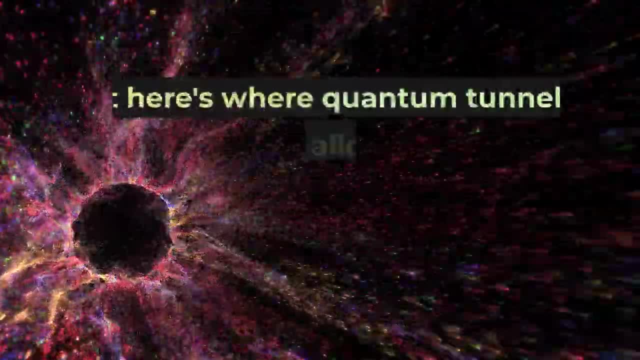 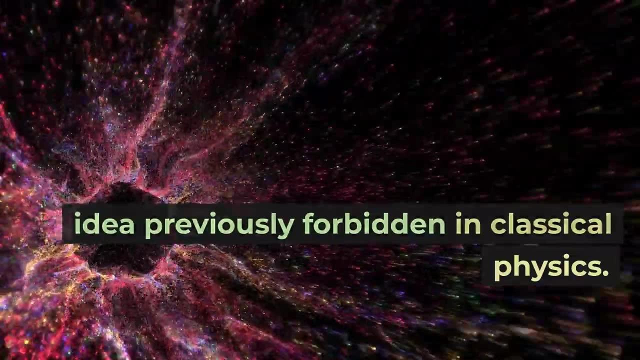 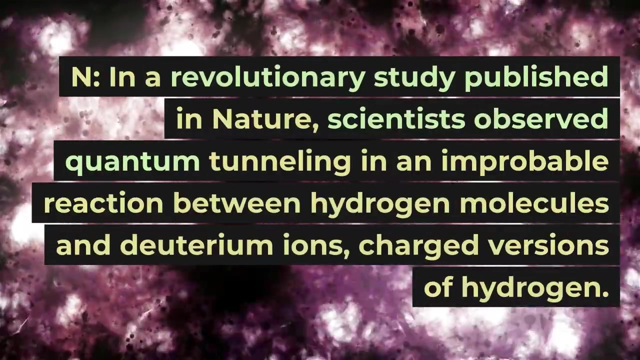 molecules lack the energy to surmount the bumps. But here's where quantum tunneling enters the scene, allowing particles to tunnel through energy barriers- an idea previously forbidden in classical physics. And in a revolutionary study published in Nature, scientists observed quantum tunneling in an improbable reaction between hydrogen molecules and deuterium. 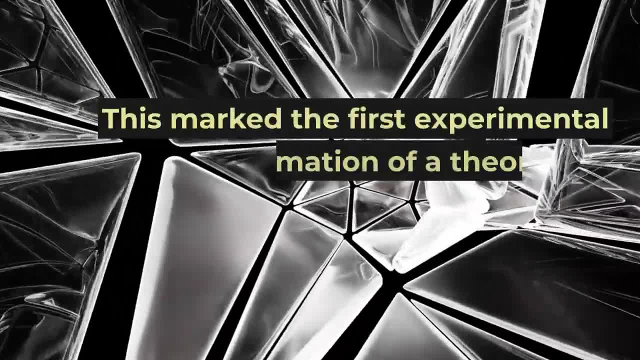 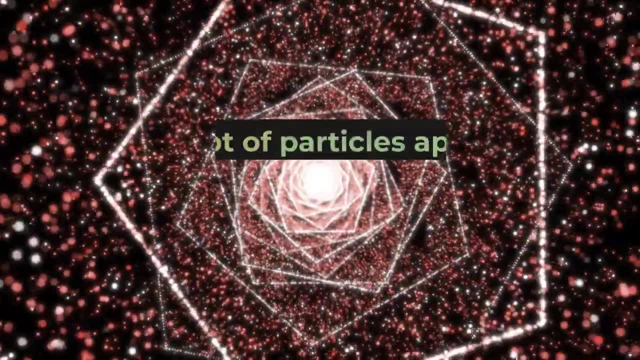 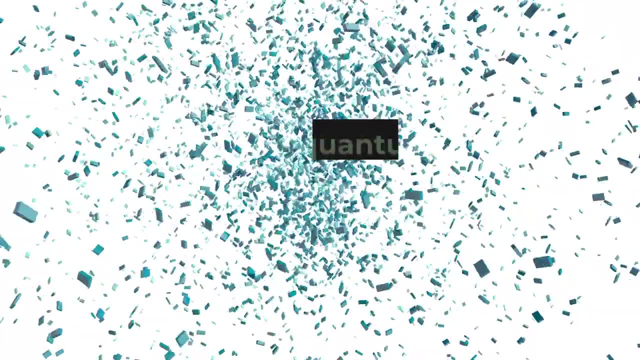 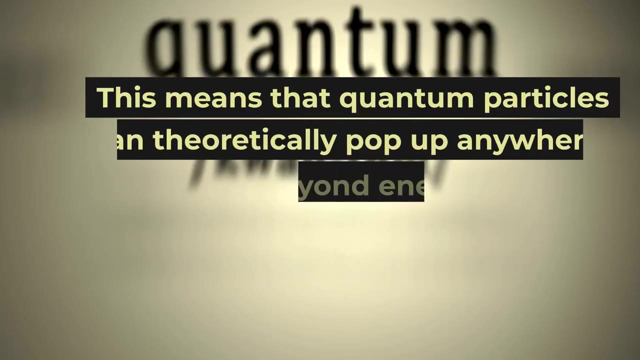 ions. This marked the first experimental confirmation of a theoretical prediction regarding tunneling in ion-involved reactions. The concept of particles appearing on the other side of an energy barrier traces back to Friedrich Hund in 1927.. According to quantum mechanics, particles exist as probability clouds extending infinitely. This means that quantum 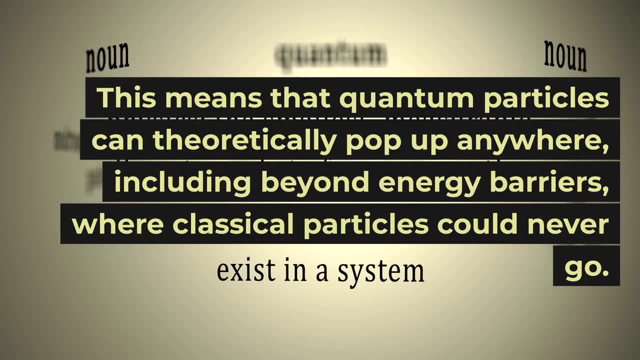 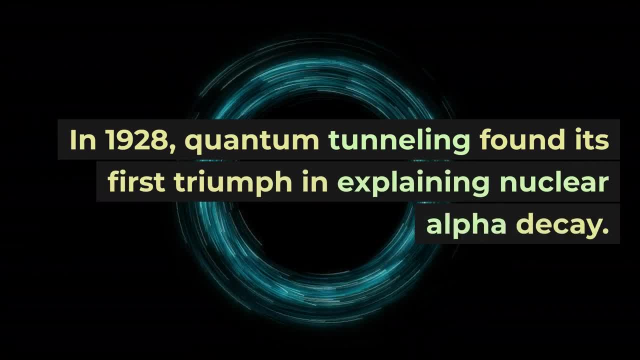 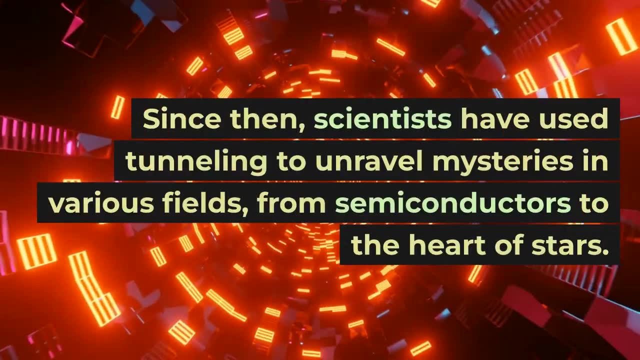 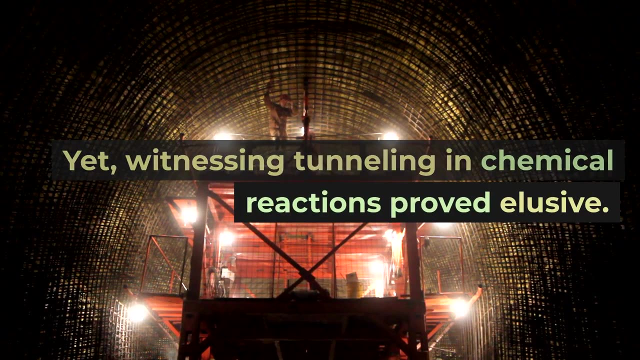 particles can theoretically pop up anywhere, including beyond energy barriers, where classical particles could never go. In 1928, quantum tunneling found its first triumph in explaining nuclear alpha decay. Since then, scientists have used tunneling to unravel mysteries in various fields, from semiconductors to the heart of stars. Yet witnessing tunneling in chemical reactions, 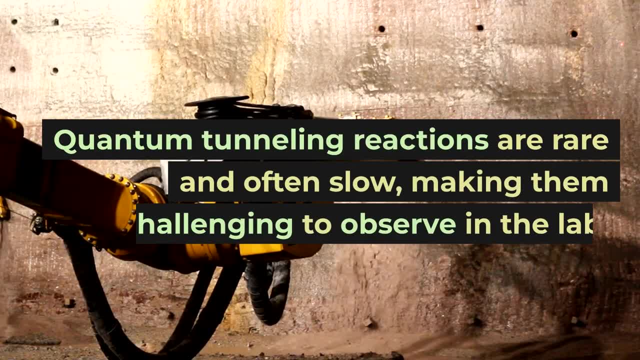 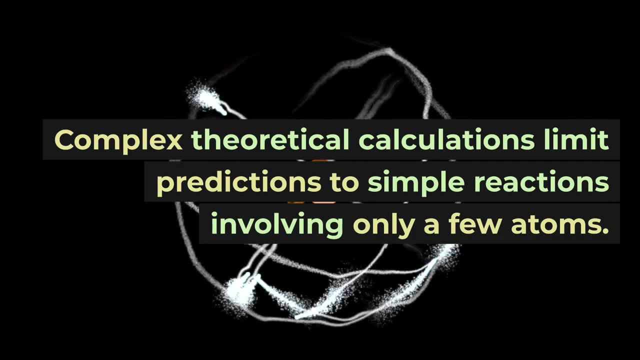 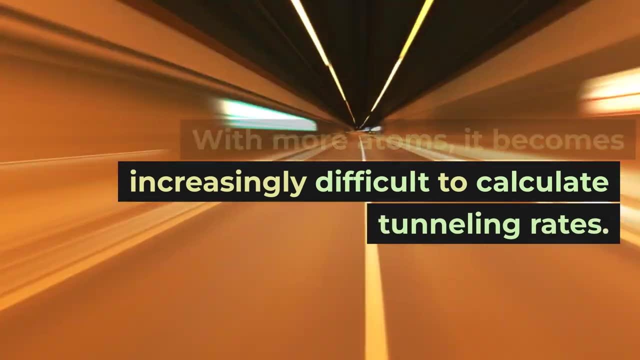 proved elusive. Quantum tunneling reactions are rare and often slow, Making them challenging to observe in the lab. Complex theoretical calculations limit predictions to simple reactions involving only a few atoms. With more atoms, it becomes increasingly difficult to calculate tunneling rates. The reaction chosen for this study between hydrogen gas and deuterium. 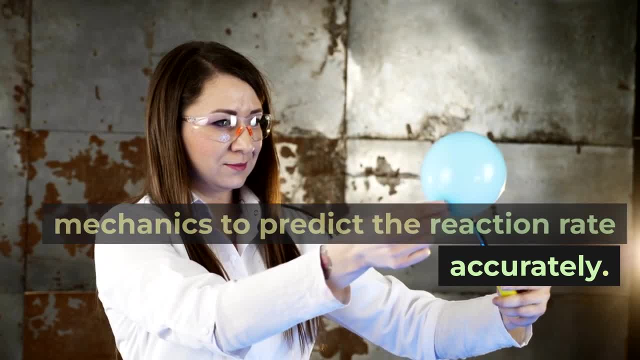 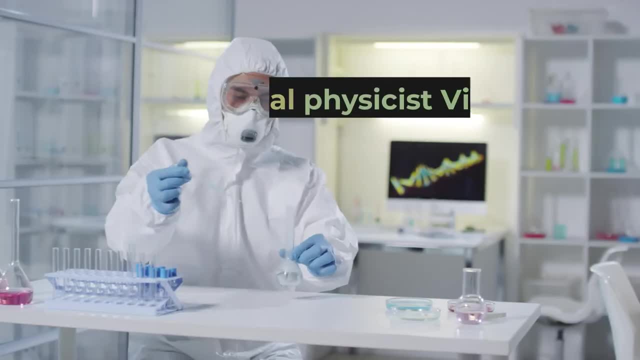 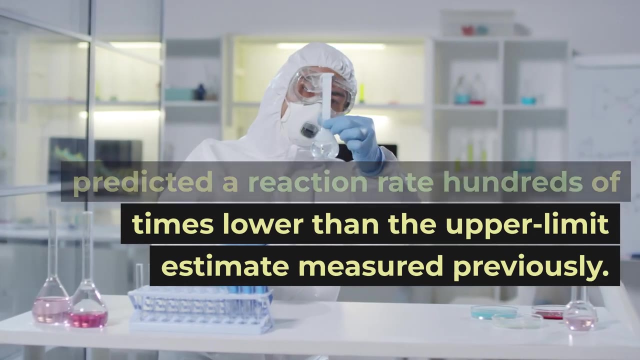 ions is simple enough for quantum mechanics to predict the reaction rate accurately. This is why the team selected it. they could finally validate theory with reality. Theoretical physicist Vyacheslav Kakoilin and his colleagues predicted a reaction rate hundreds of times lower than the upper limit estimate measured previously. The initial discrepancy- 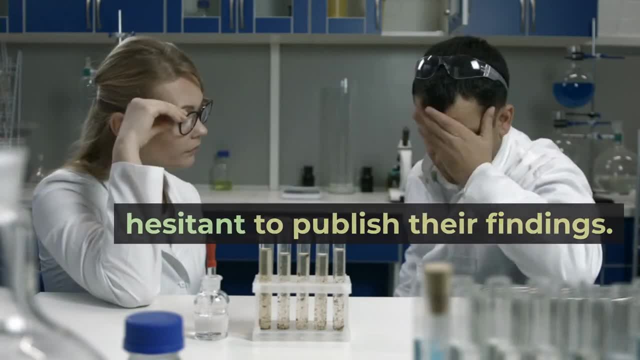 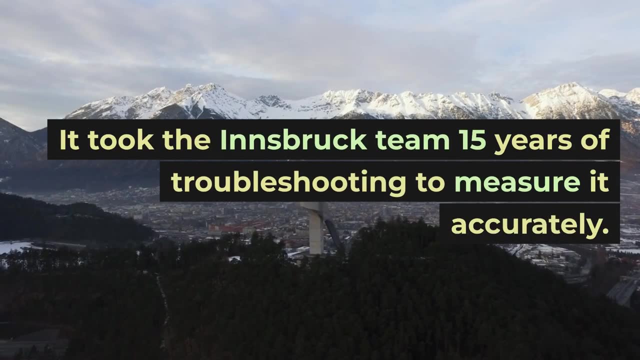 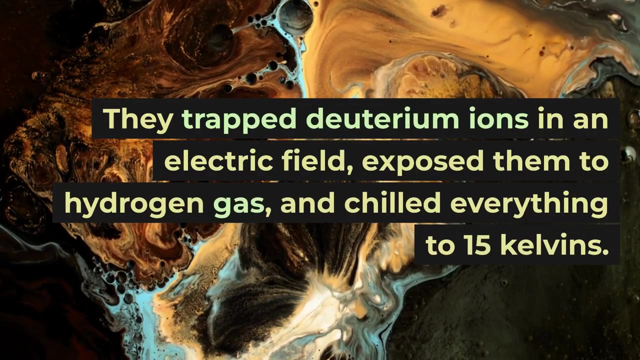 between theory and experiment left them hesitant to publish their findings. The root of the problem lay in the reaction's exceptionally slow rate. It took the Innsbruck team 15 years of troubleshooting to measure it accurately. They trapped deuterium ions in an electric field, exposed them to hydrogen.